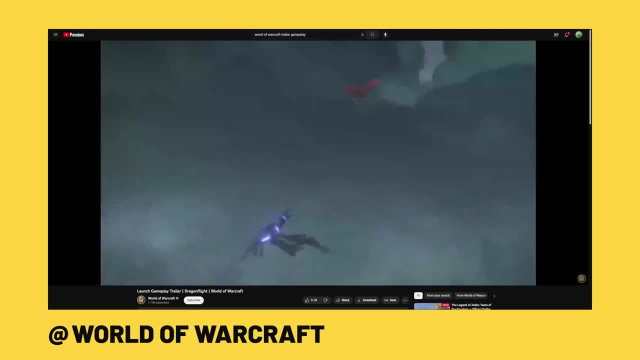 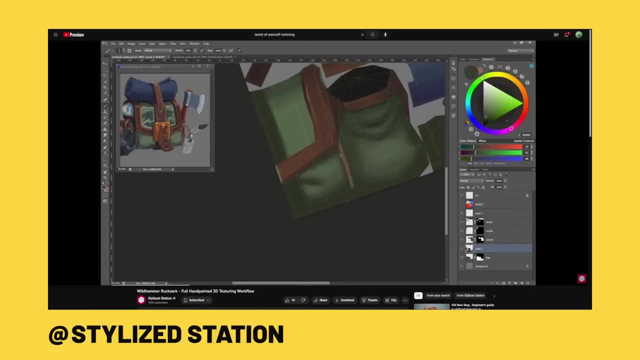 paint all the textures. It gives it a cool, stylized, very timeless look. However, yet again, unless you're doing a smaller scene, this may not be the best option for an individual artist. So enter method number three, which we'll be using as our solution, And this comes: 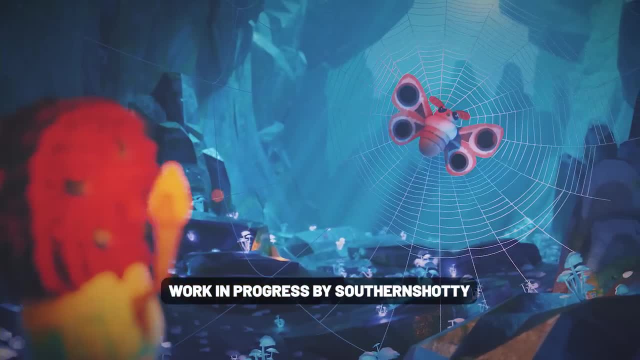 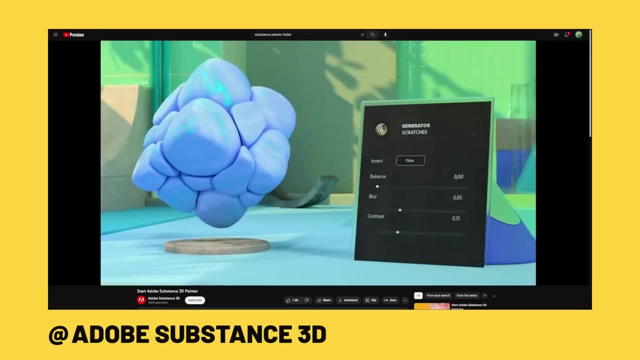 courtesy of game dev studios popularizing this method over the last few years, And it comes with things in terms of generators and automatic maps. So what does that mean? It means that the texturing software takes into account things like edges, materials, normers and inclusion and can use. 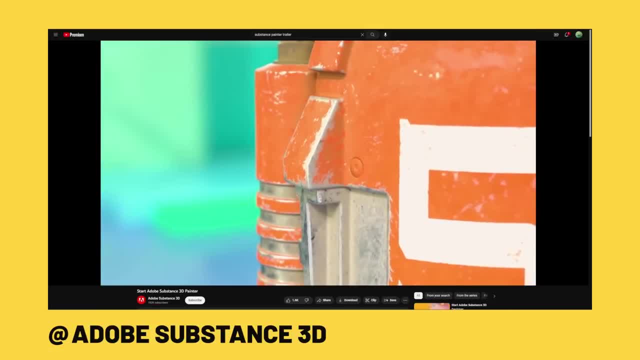 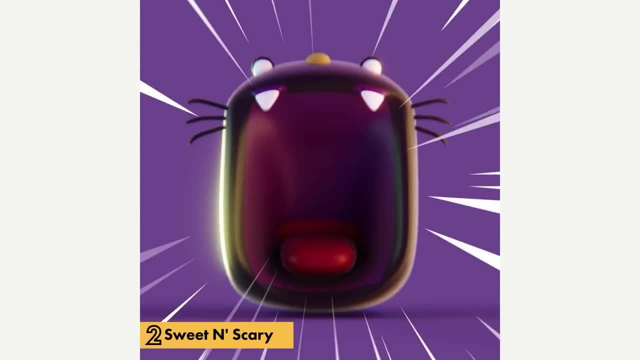 all those to mix things into the roughness map, into the base color and really add story to your texture. Well, adding story to your texture is a large role in what differentiates a good texture from a bad texture. So how do we get? 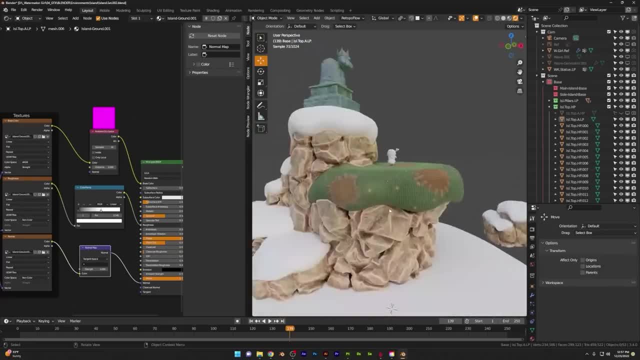 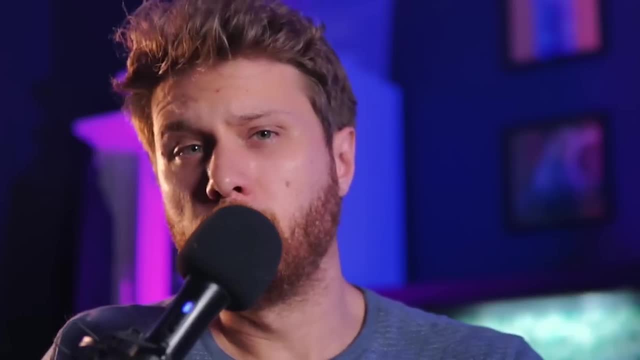 This inside of Blender. Well, the good news is that apparently it's in development at Blender to add more of these within the material tree, but you probably click this video because you want a solution now. So let's look at three main types of generators that occur in substance: painter that. 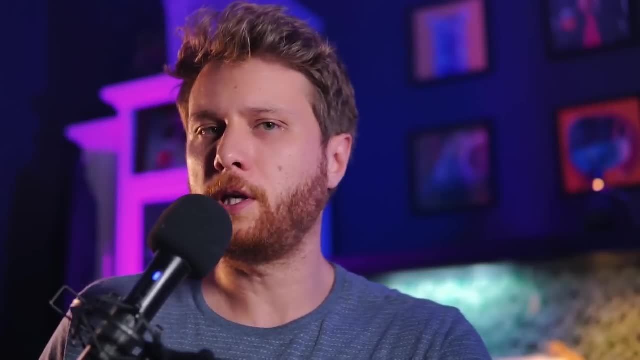 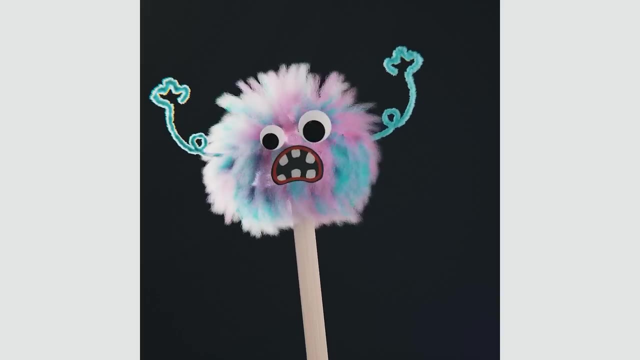 for the most part, can get us most of these results in Blender, And we're going to look at how to create each of those generators. And, for those of you who stick around to the end of the video, I'll also be showing you where you can get some free materials and resources to help you do this. 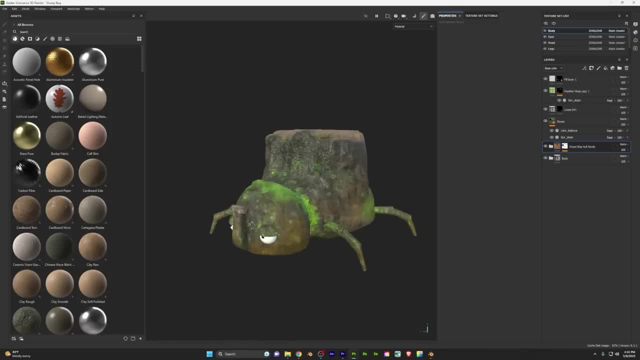 stuff a bit easier. But for now let's dive into method number three, Method one, So method number one: when using a tool like Substance Painter with generative add-ons, it will take into position into account of some of the add-ons. So for example, in this bug I wanted 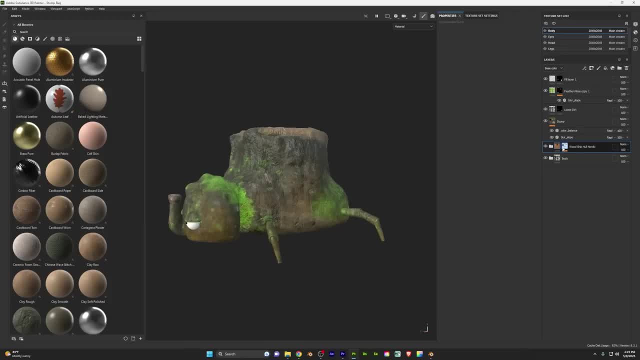 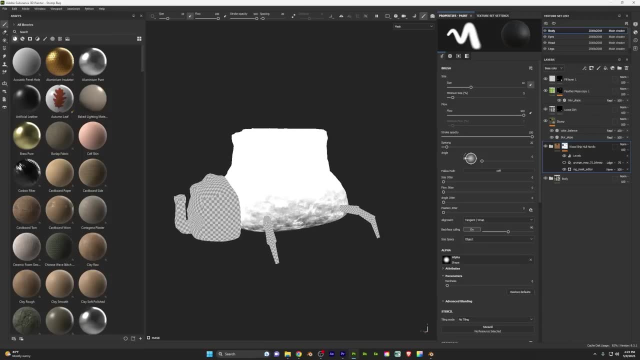 the bottom to be more rough than the top in terms of color. If you go ahead and look at the mask that has been generated here, you can see that we're getting that gradation from the bottom to the top. This is going to be the simplest of the three, So let's dive into Blender and look at how we can. 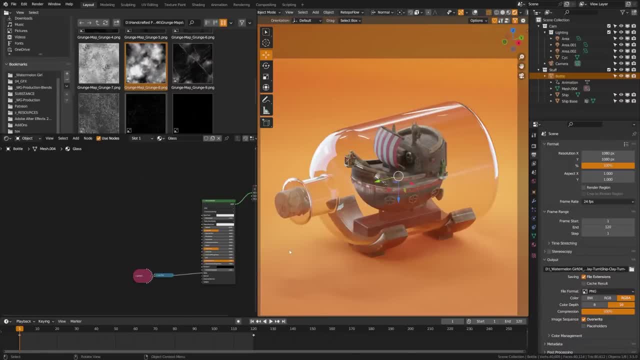 recreate this. This makes for a great example for a positional generative map, Because if this was a real life bottle, there would likely be dust and other grunge kind of collected down here where it is harder to clean. So let's look at how we can go about doing that. 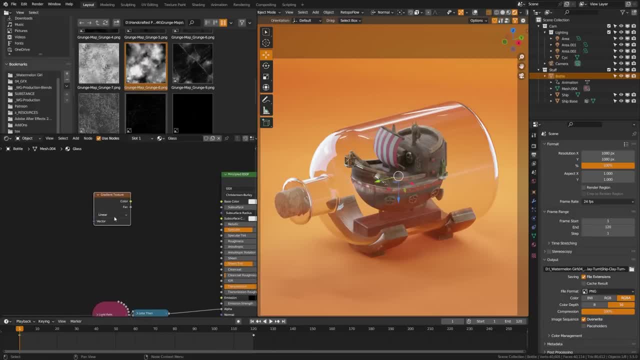 Let's go ahead: hit shift A here and we'll add a gradient texture. I'm going to leave this to linear and I have node wrangler nabs on, So if I hit control T, that will go ahead and add a generated coordinate. Let's go ahead: drug this color off here, plug this into a color ramp with a factor. 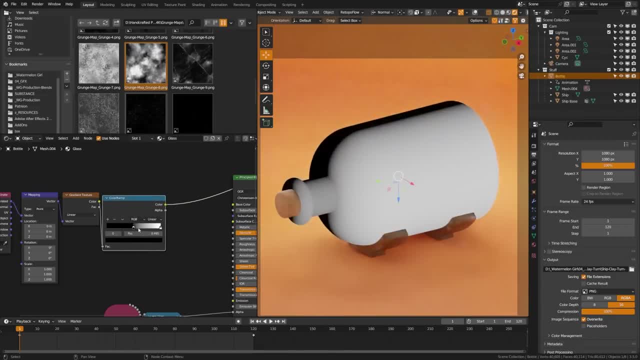 and then I'm going to hit control shift T so I can see what I'm doing. I see that my gradients coming from the wrong direction and it's a bit harsh, So I'm going to go ahead: rotate the Y 90 degrees. 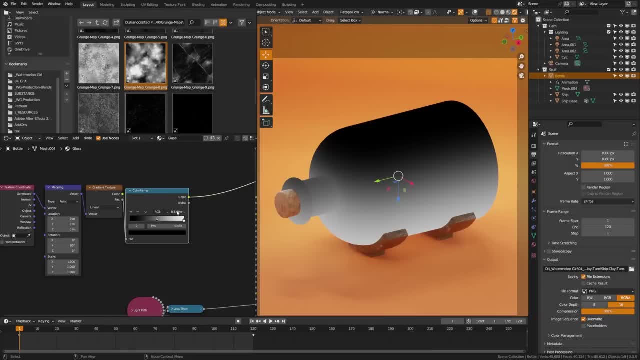 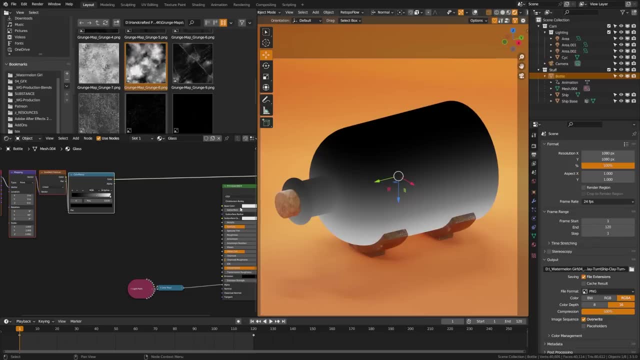 and then I'm going to take this linear here and set this to B spline and get us a more gradual fall off. Perfect, That's about how much grunge. I kind of want to ride up the edge of the bottle here. But if we go ahead and switch back to render view and we plug this into our roughness, 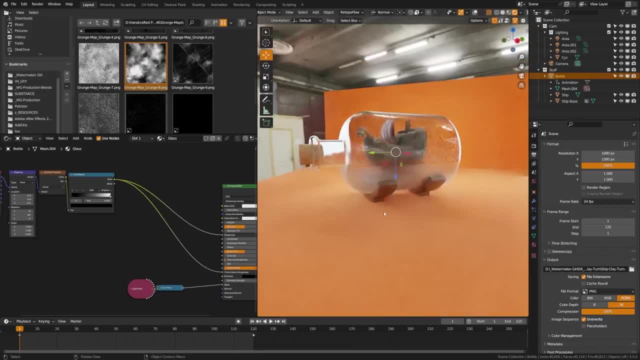 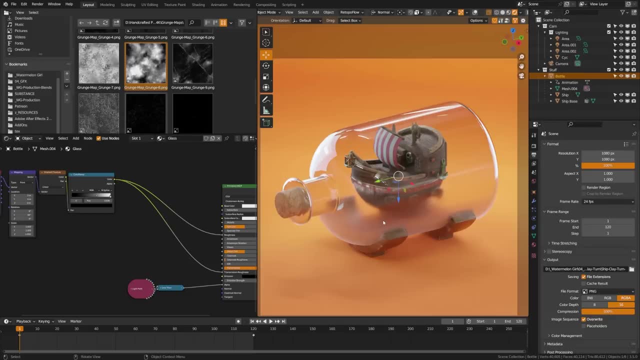 and our transmission roughness, you can see that it's just giving us kind of a frosted glass fall off, And that's why oftentimes, whenever you're using a generative map, it's a good idea to introduce textures or grunge textures into it. This is actually something that 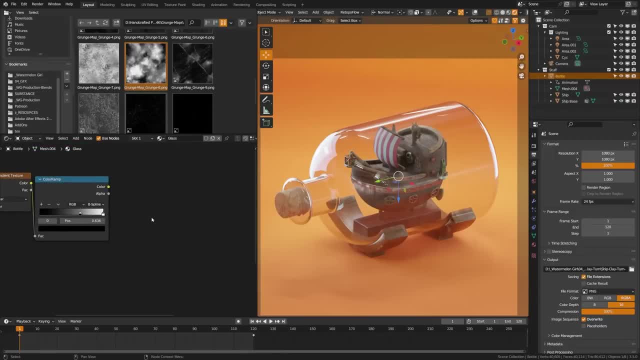 substance does automatically on all of its additive generators. So I'm going to go ahead and grab a grunge map I have up here. I'll give you a free one at the end of the video, but for now let's just kind of walk through this process. We're going to go ahead, add a mix factor here. 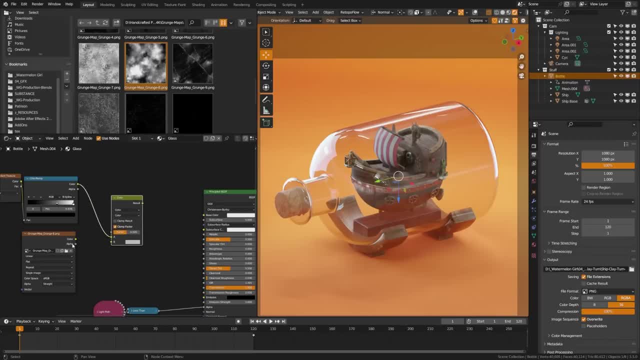 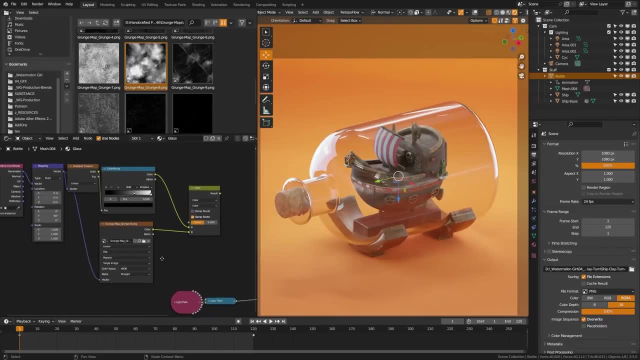 and we're going to go down here to mix color. Great, We'll leave that plugged into the top. We'll plug this into the bottom. We need to make sure that our grunge map has some generated coordinates, so we'll plug that into the vector and let's go ahead and see what we 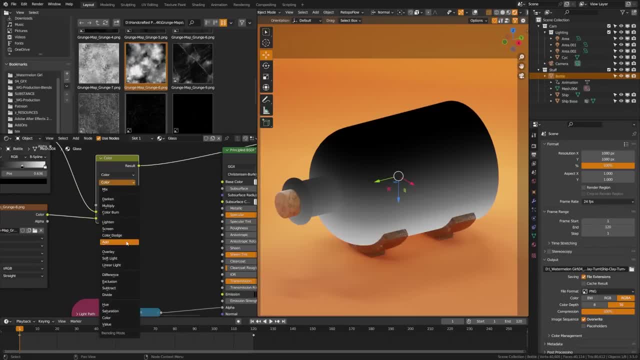 have. You can see that right now we're not able to see much with this kind of color drop down. so let's go ahead, change this to multiply and now you can see that our texture is coming through. and if we turn this up, you can see that we're starting to get a bit more interest there. You can also 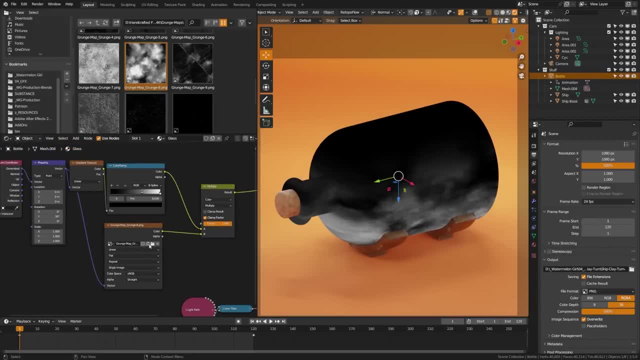 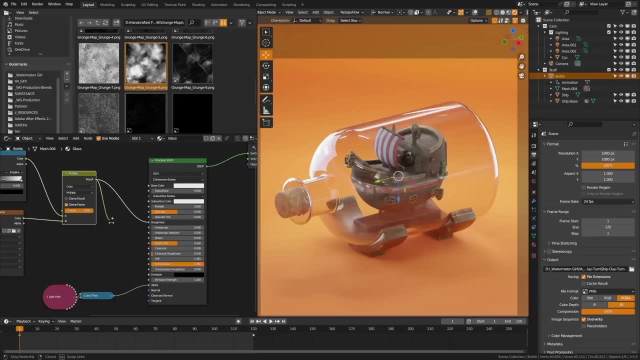 play ahead with these object coordinates if you want, but I'm going to leave mine on generated for now. Perfect, let's switch back to this view and we'll go ahead and plug this into the roughness value, and then we'll also go ahead and plug this into the transmission roughness and you can see. 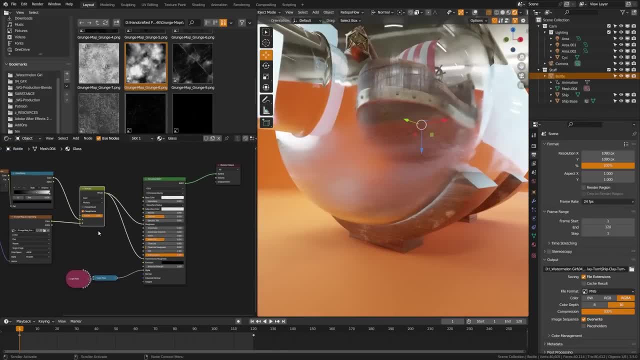 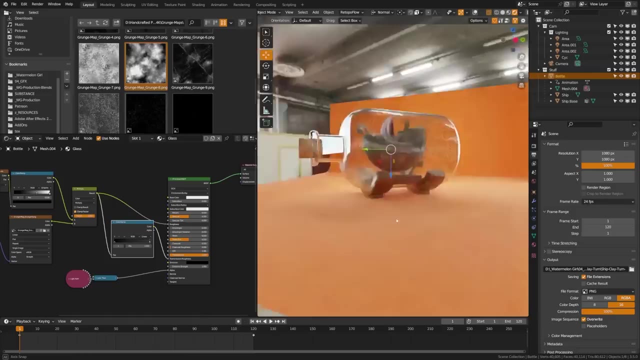 that now we're starting to get some results. You can also go ahead and add additional color ramps to help control how much it affects these various areas. So by grabbing this one and lowering the white value, you can see that it is not affecting it as much, and I start to get a more kind of 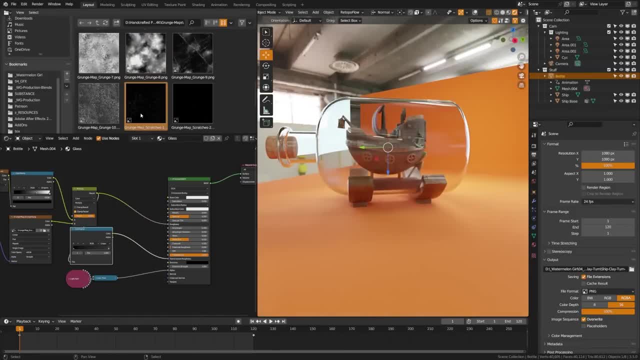 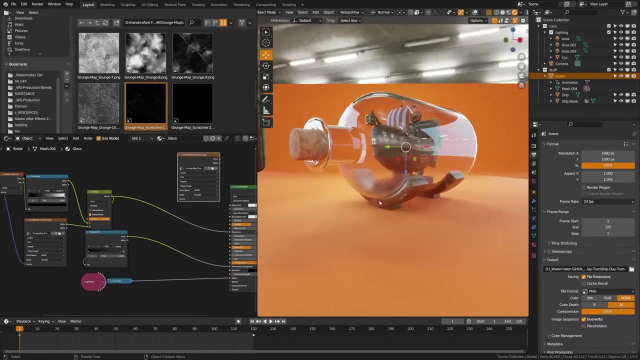 natural fall off. Now another thing you can do is go ahead and add kind of grunge maps over on top of everything. This is also something that I like to do. So generally what I'll do is I'll go ahead, add a generative layer or an. 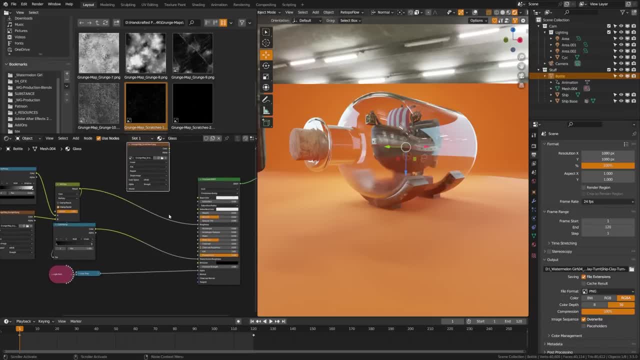 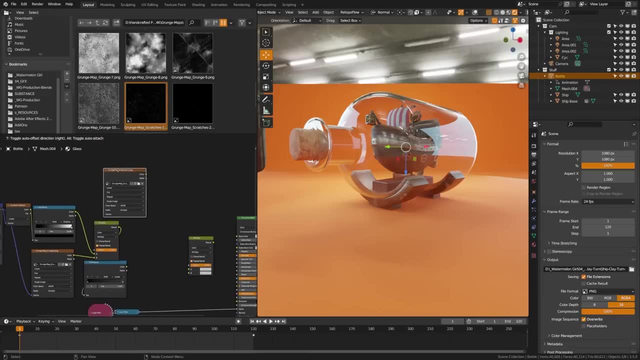 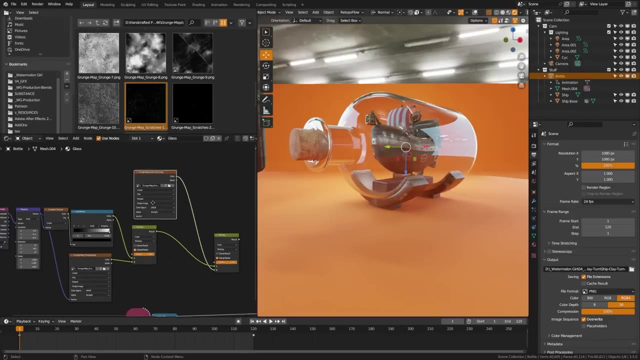 automatically generated layer, and then I'll go ahead and add a texture on top of everything. So let's see what that looks like. Let's go ahead and add this right here. We'll take this node over and what we're going to do is plug this into the top layer there and we'll plug this into the bottom. 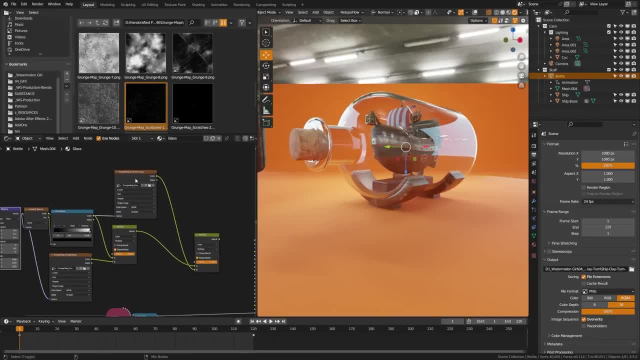 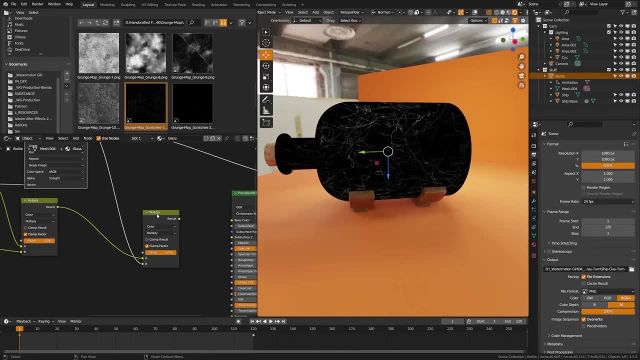 layer. We'll go ahead and add this right here. Let's see what this grunge map looks like. We can see that this is kind of giving us some scratch. It's overall which could help add to the realism. So let's go ahead and look at how this is mixing. 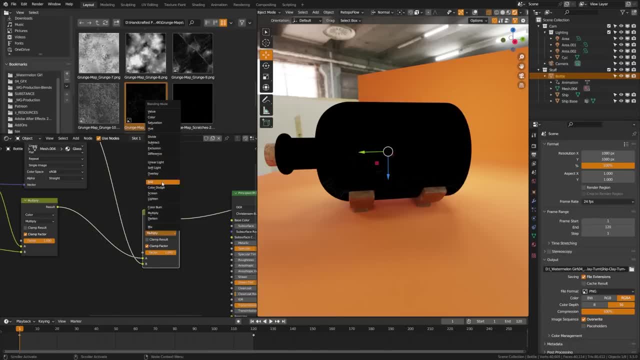 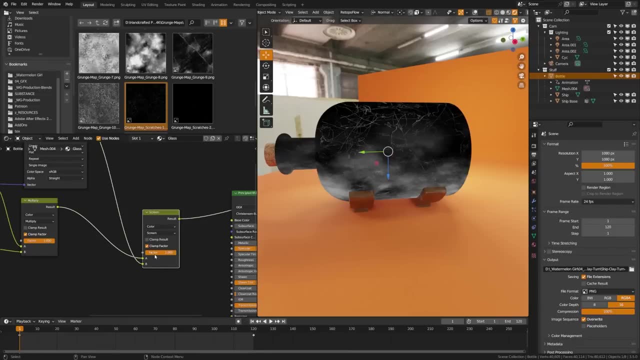 You can see, right now we're not seeing much with the multiplying. that's because in this case, we want to set this to screen. Now, if you don't know, screen will basically filter out all the black in your image and put it B on top of A. Multiply will take all the black of the image and keep it and put it. 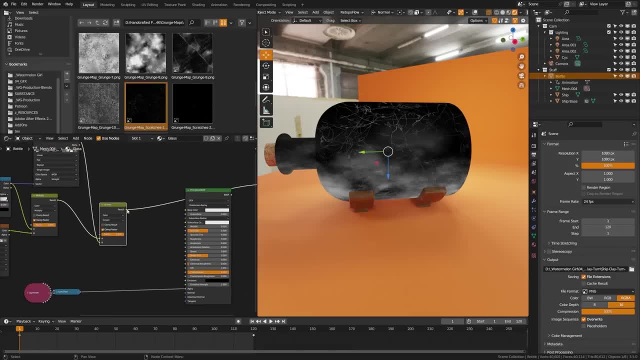 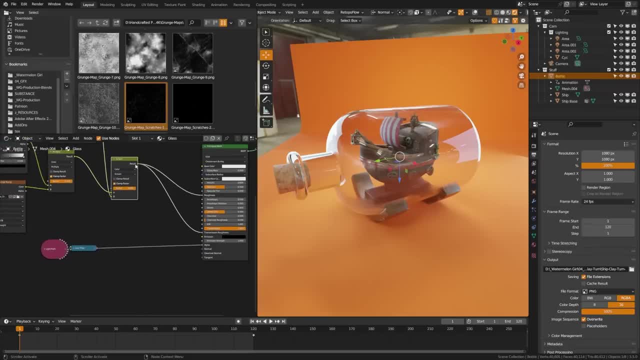 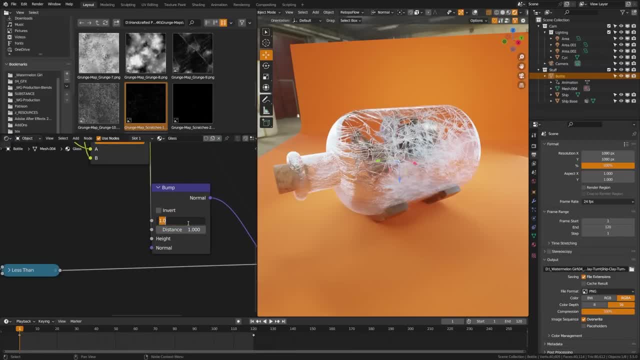 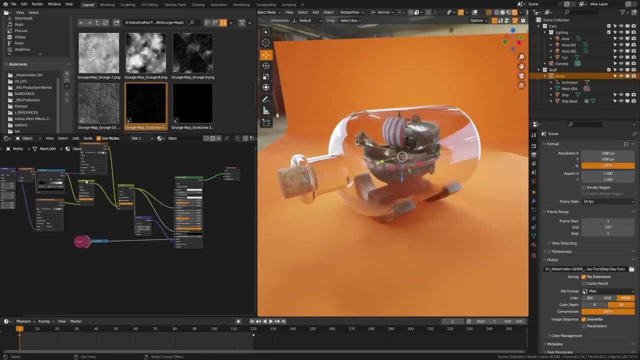 the normal, and this can also help add some realism at a much smaller number. So let's go ahead, do point zero, one, five, and you can see that now we're starting to get some indentations in there. So by using this kind of gradient to drive our position, you can end up adding a lot of realism. 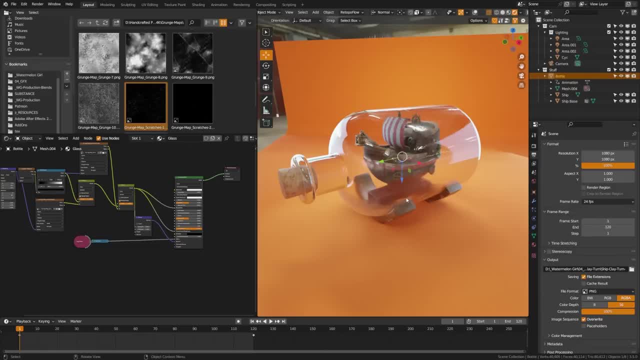 Another great example of how to use this would be if you used moss growing up from from the bottom of a tree, dust growing on the bottom of a dresser, or you can imagine some other scenarios as well. Next up, let's take a look at how we can use things like ambient inclusion. 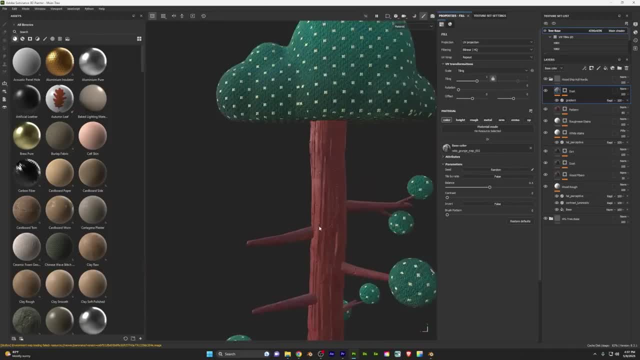 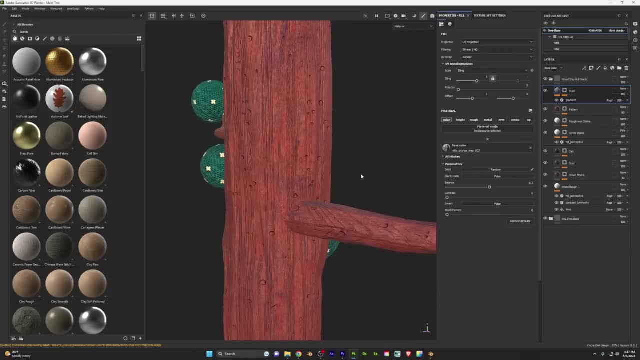 and kind of curvature data in order to kind of better create a more realistic texture. So here you can see that I am using that to go ahead and insert some of those colors into the cracks. here You can see some of the generative ones I have here that are kind of detecting the cracks and 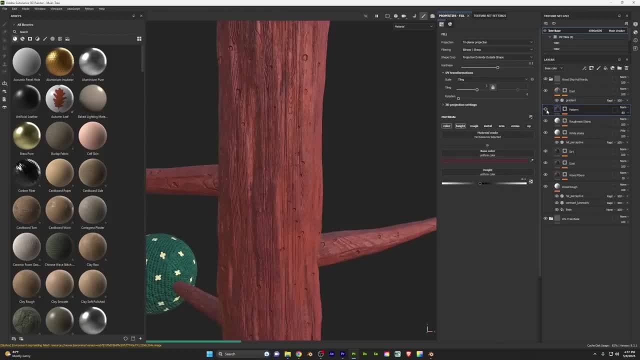 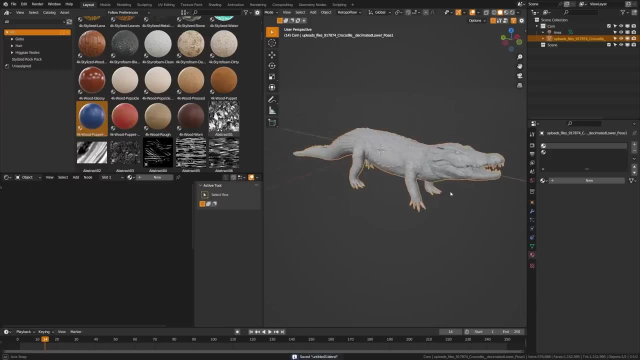 inserting kind of that colored pattern there. If I go ahead and switch over here and turn that on and off, you can see how big of a difference that is making. Let's look at how we can achieve this in Blender- Okay, great. So for this example we're going to be using this- really detailed. 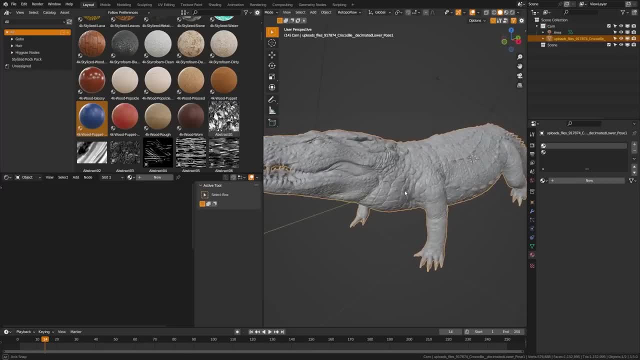 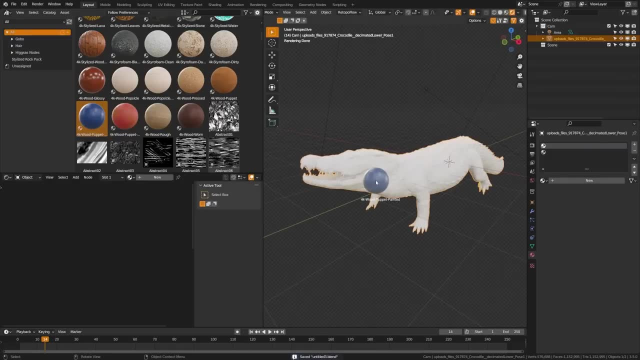 alligator skull. So let's go ahead and drag a material on it and look at how we can get some of that cavity information out of it. So I'm going to go ahead here, switch to rendered view and let's say that we want to make this look like it's kind of a painted wood sculpture. So we'll go. 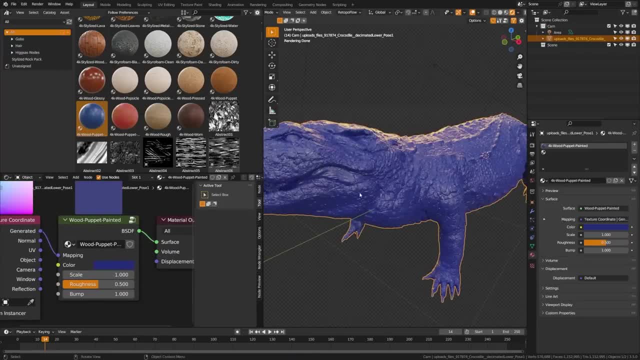 ahead here. switch this over to generated and you can see that it's kind of a painted wood sculpture. So we'll go ahead here. switch this over to generated. that that's looking good. We got kind of our painted wooden alligator. Now let's add some. 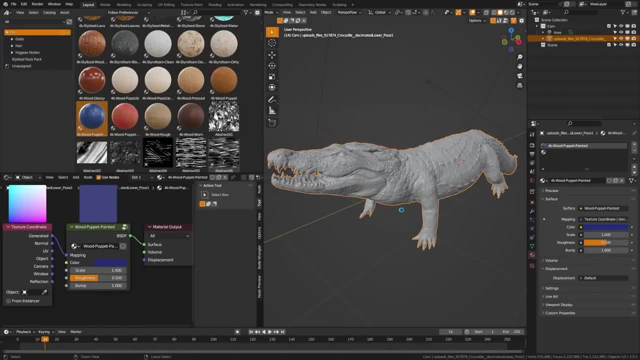 paint wear based off of the cavity information. So it's actually quite simple. What you want to do is you want to grab your object, hold tab and switch over to vertex paint mode. Then what you're going to do is you're going to come up here to paint and you're going to come down here to 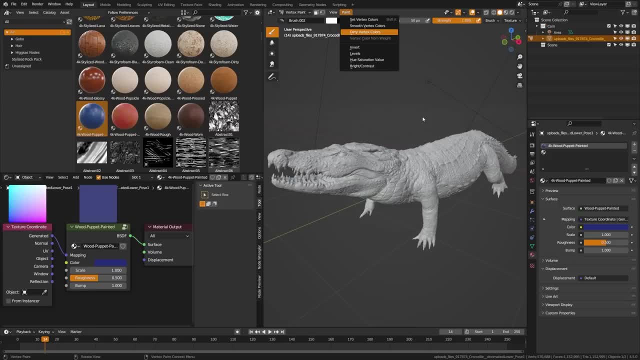 dirty vertex colors. Click that. Depending on the complexity of your geometry, it may take a while to load, but once it is done loading you will see that option appear down here And then, once that's there, you can go ahead, click that up and begin adjusting. 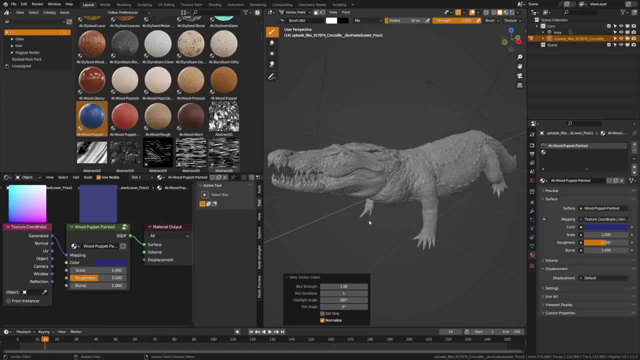 the parameters Here. what I really want to do is have just only the dirt visible. So by clicking dirt only, what it will do is kind of get rid of this wash across the whole thing and show me just the dirt. Great, And now I have that information. You can see how that's kind of appearing in the cracks and where 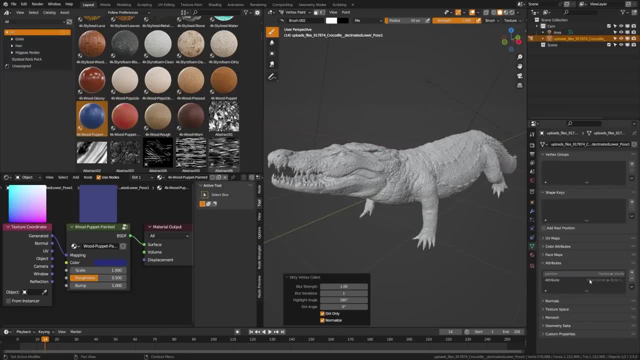 that is saved is actually over here under your mesh data and the attributes tab You can see we have that down here, So we'll go ahead and call upon that in our shader. So let's switch back over to the object mode and I'm going to switch into rendered view so that I can see what I am doing better. 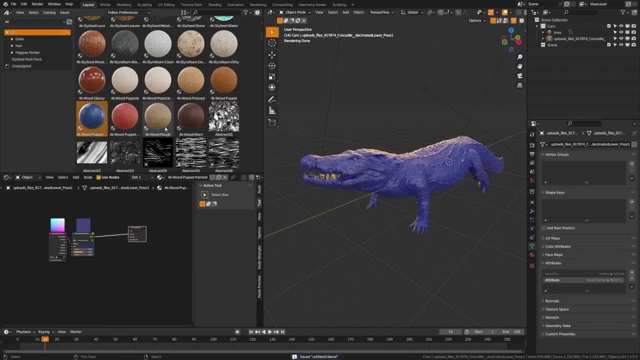 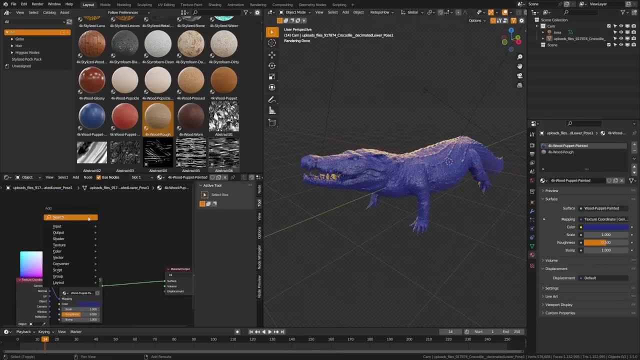 And then I'm going to go ahead and just grab another material in the scene. I want to go ahead and do kind of wooden rough appearing underneath there. I'm just going to go ahead, drag that in there so I can quickly access it. Go ahead, here I'm going to search for wood rough. I'm also going to generate this mapping here. 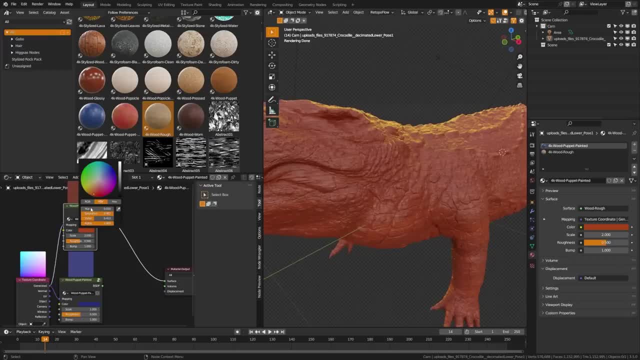 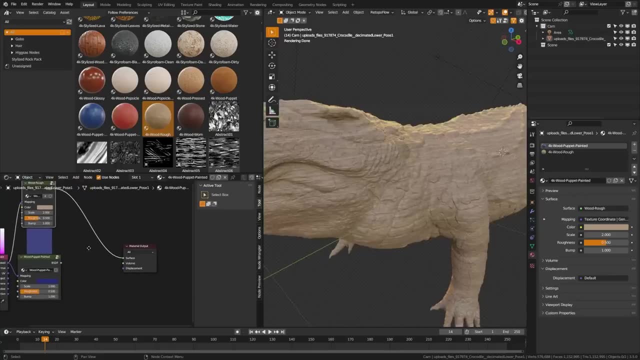 and plug this in just to see what this is looking like. Great, I'm going to go ahead and pick a brighter wood there so that it stands out a bit more Perfect. Now what I want to do is mix these two things based on that crevice data that I have, So we can call upon. 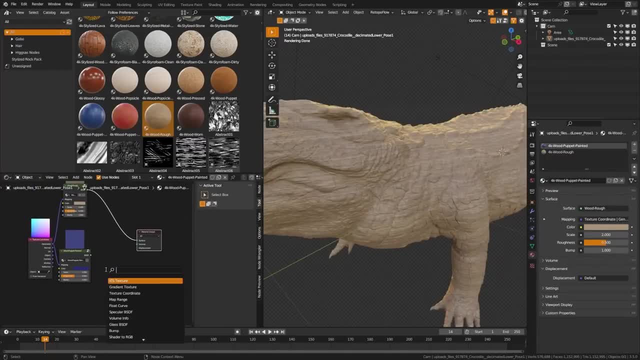 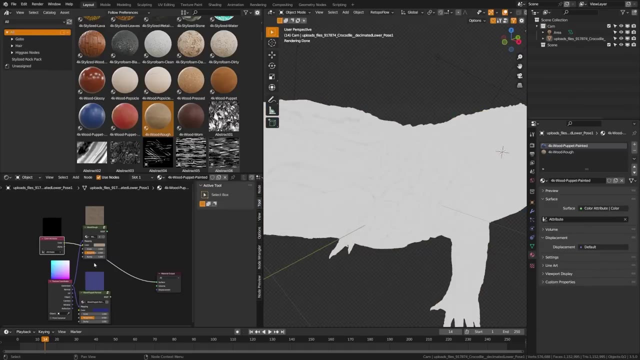 that in here with the attributes. So we'll go ahead, search, look for color attribute, click that, and you should click here and you'll see that attribute appear and you can name that whatever you want in that mesh data. I'm just going to go ahead and leave that for default now, But let's go ahead and look at what this color data. 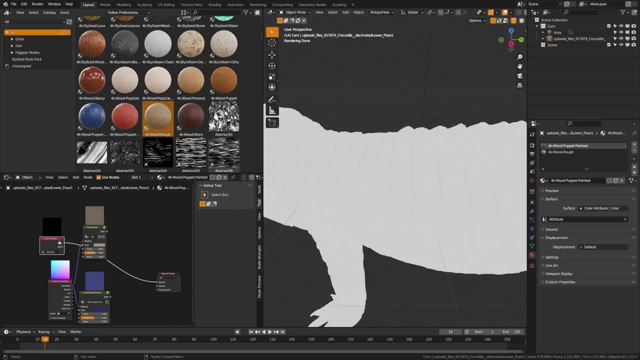 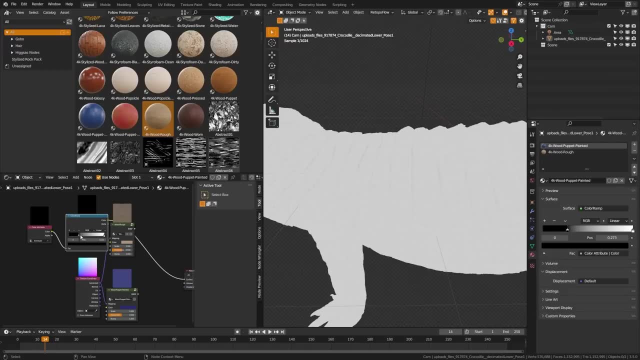 is showing. You can show that we're starting to get kind of all this data in here And let's go ahead and add a color ramp to this. We can even crush this a bit and make that a bit more prominent. Perfect, So now you can see. 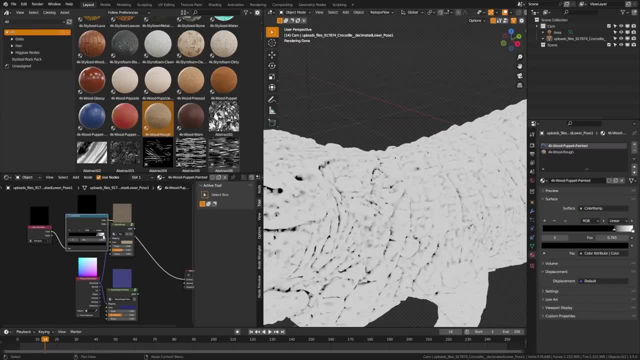 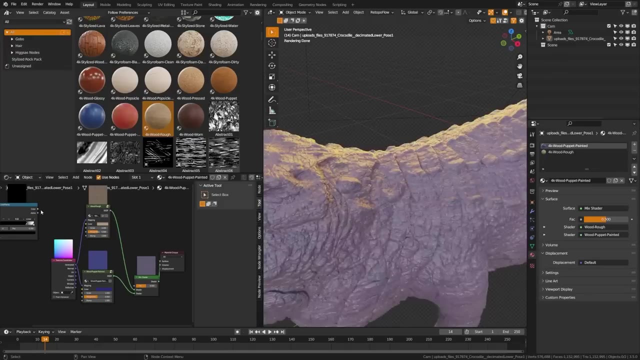 that, where all those cracks are, we're starting to get a bit more black. Perfect. Now what we want to do is go ahead and use a mix shader between these two, And then we will go ahead and plug this data into the factor here, And you can. 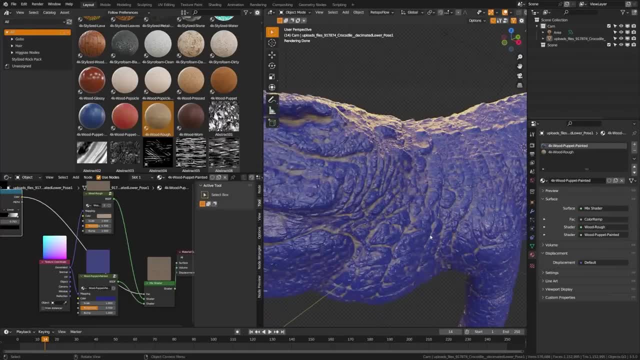 see that we're starting to get a bit more black. Perfect. Now what we want to do is go ahead and use a mix shader between. see that where all those cracks are, we're actually starting to get a wear and tear away, where the paint is kind of chipping. 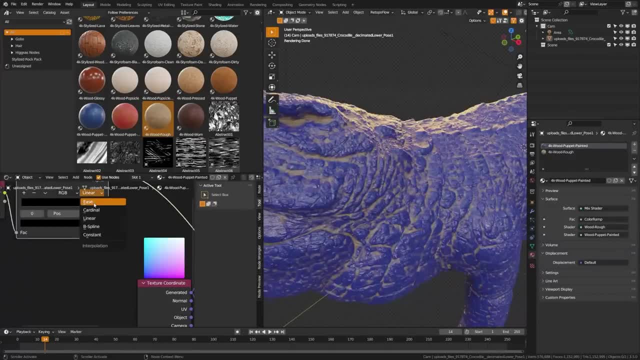 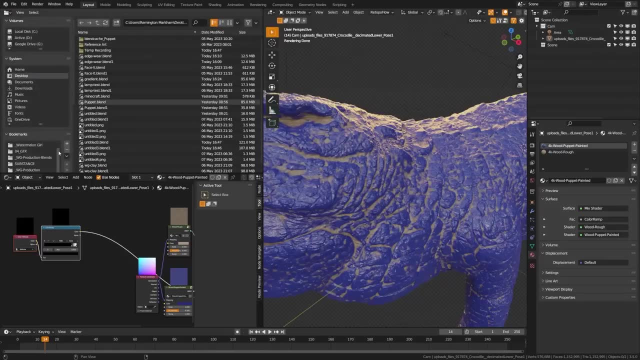 away as it kind of gets weathered over time, And we can go ahead and increase that if we want a bit, And then, like before, we can actually go ahead and also just add some kind of various grunge on there as well to further kind of assist the effect. So just as a 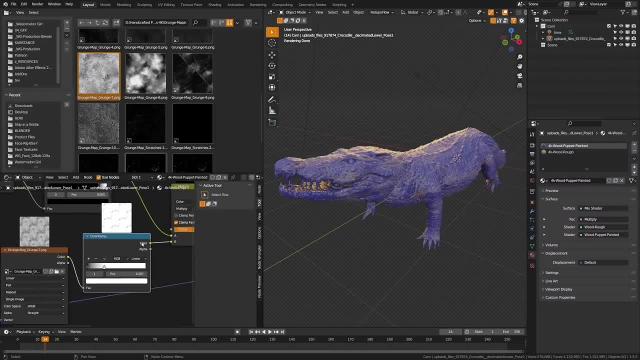 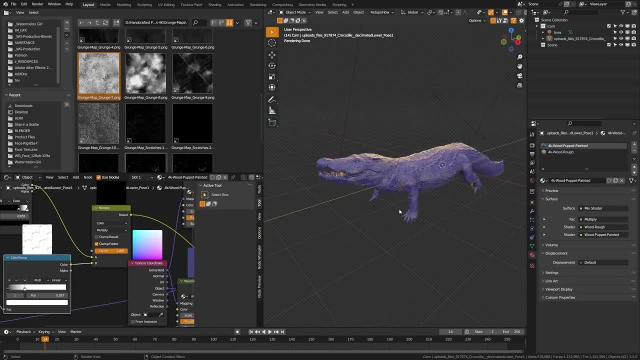 quick example here. you can see that I've taken a grunge map, plugged it into a color ramp, multiplied it over there and you can see that now it's adding kind of additional wear and tear and peeling to our object. So that's one way you can go about accessing crevice data as well. Another way, although not as 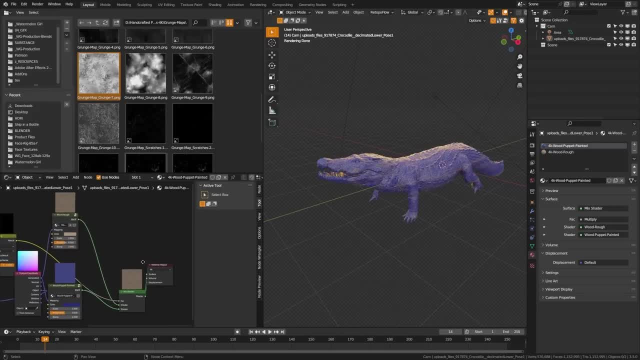 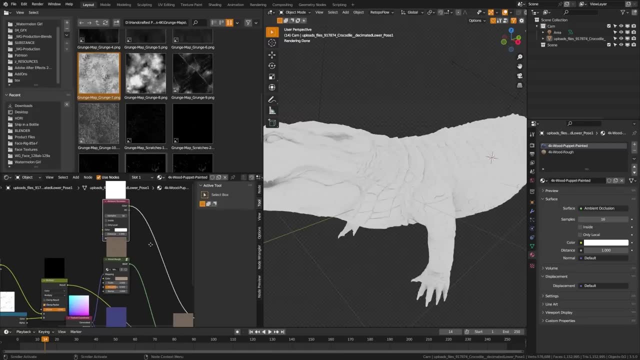 accurate- it will load quicker and be a bit simpler to implement- is you can actually use the ambient inclusion node. So if you go ahead and see what our ambient inclusion is doing, you can see that it is naturally kind of getting all those crevices. So we can go ahead. take that. 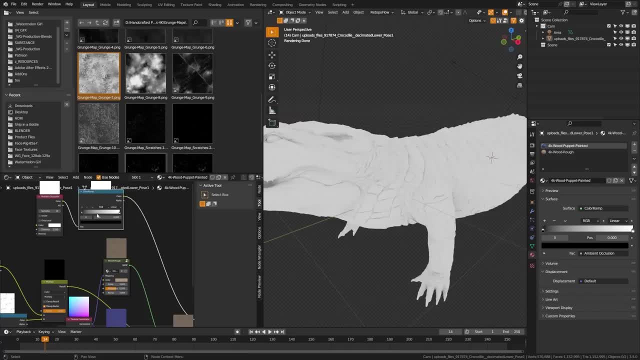 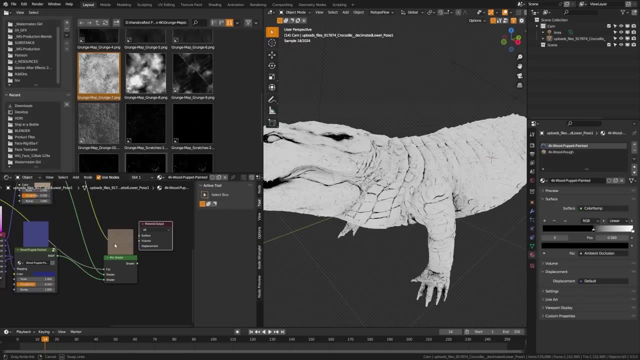 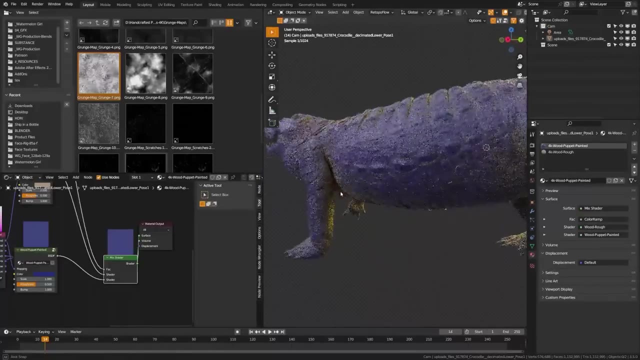 ambient inclusion, color. drag a color ramp on it, crush that down And you can see that it gives us a very similar result, but it's not those crevices. So this is a very similar result, but it's not really being deployed here. Now let's take a look at the edge detection. Let's look at the cavity detection. So if you go ahead and click on the value, 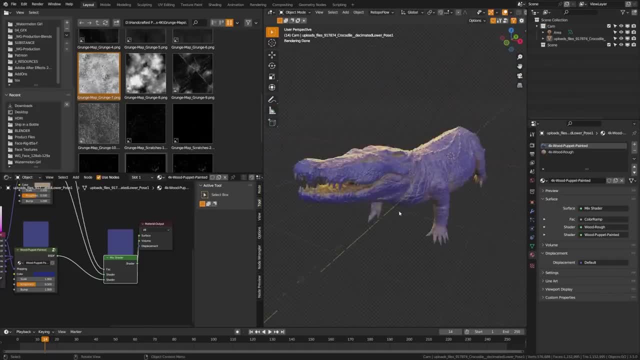 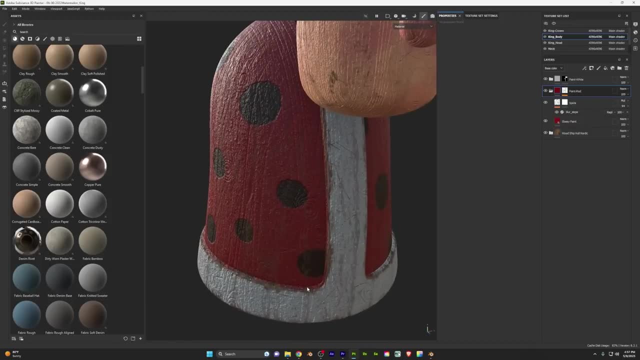 areas it's pop up as a bit slower and a bit more accurate, although a bit speedier and a little less accurate. So we go ahead, plug this into the factor and plug then in there And you can see that that is also giving us kind of some wear and tear and even getting in things here like on the armpit, where it would. kind of naturally wear off over time from friction. Now, lastly, let's take a look at edge detection. This is kind of like the cavity detection, except this is more along sharp edges of the object. So if I go ahead here and click, 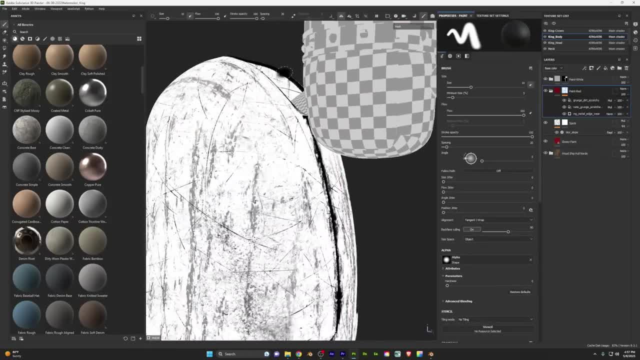 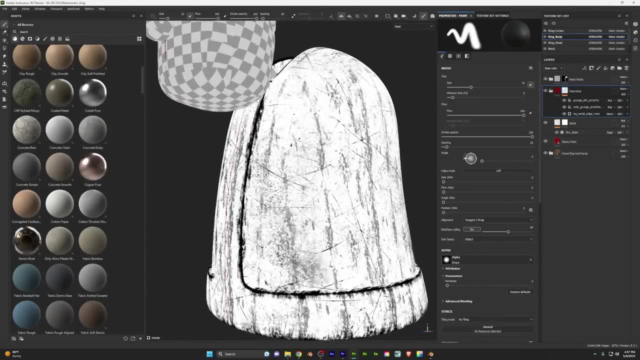 So if I go ahead here and click this, you can see that wherever there is a harsh edge, that the paint is kind of worn off. So this edge detection is actually pretty simple to get in Blender. So let's take a look at that. 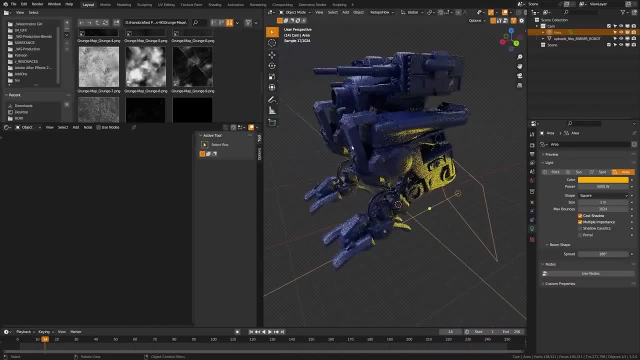 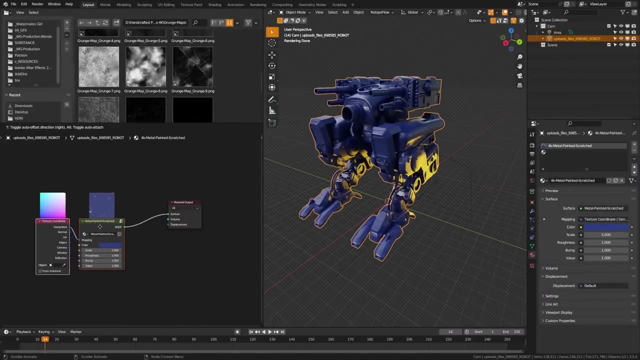 So here, I have downloaded this mech file and we're going to be looking at how we can go ahead and add some edge wear here to wear out the paint and reveal the metal underneath. Now there are two ways you can go about achieving this. 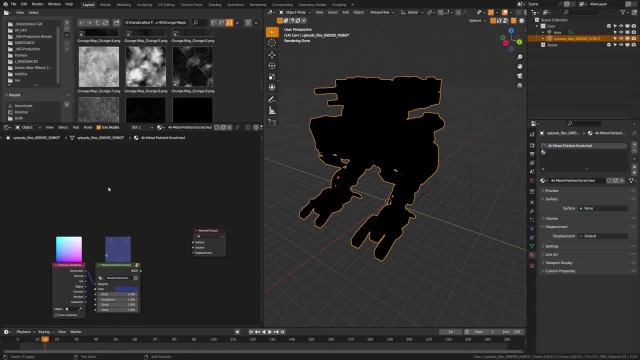 Let's go ahead, get rid of this so we can view this on our model directly. So first is, if you pull up the geometry node and you go ahead and take the pointiness value here and plug this into a color ramp factor, you can go ahead and plug this directly in. 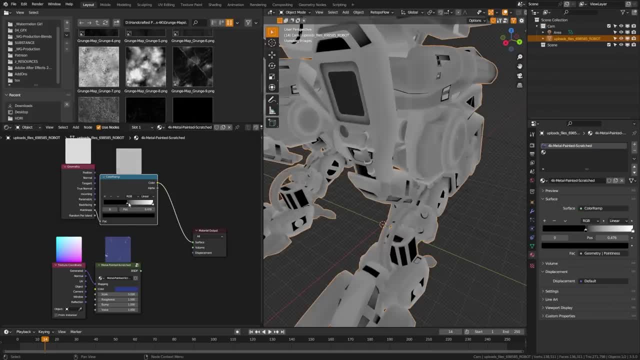 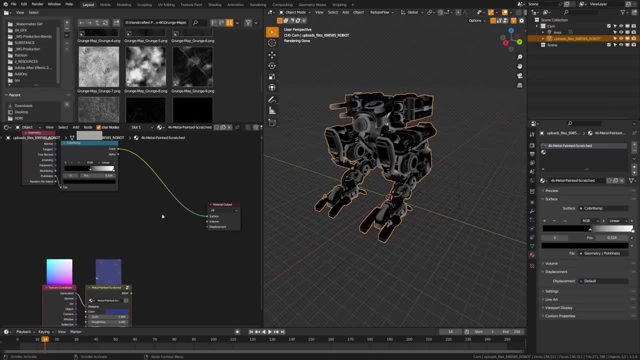 And you'll be able to see that we're starting to get some of those edges based on kind of the pointiness there of the geometry. So this is one way you can go about doing it. Another way and a more common method is using the bevel node. 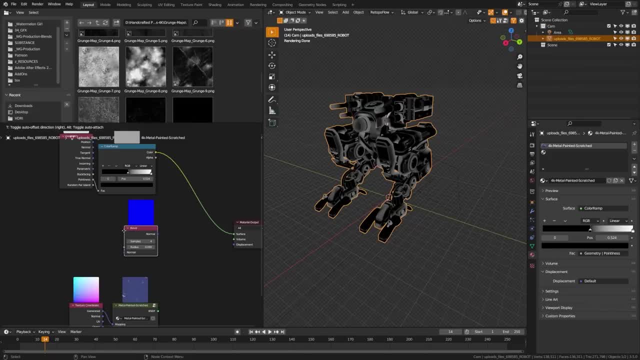 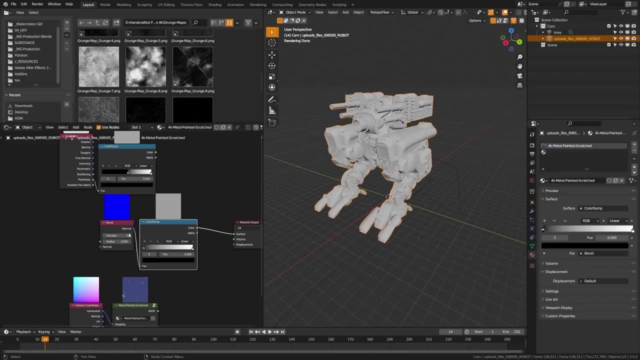 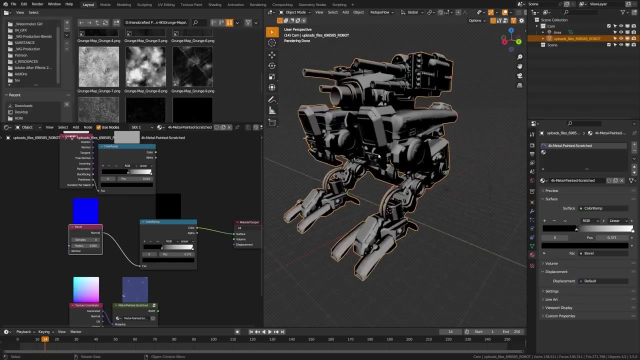 So if we'll go ahead, grab the bevel node here, We'll plug this into a color ramp factor and plug that into here. you can see that we don't really get that great of data at first because it's kind of smeared all over the object and around the corner. 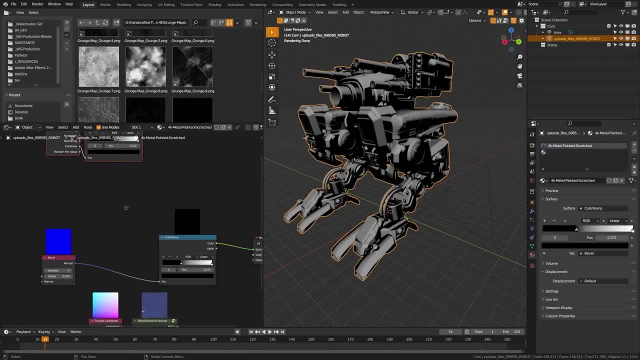 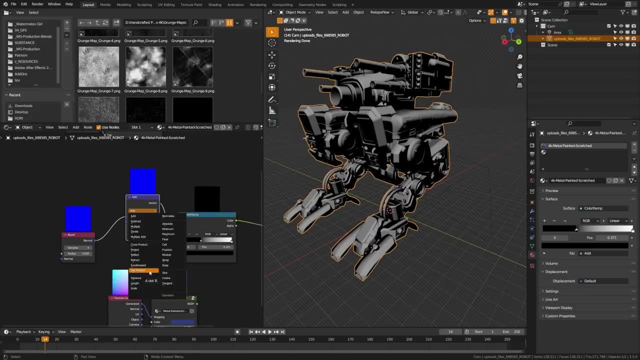 So let's go ahead and refine this a bit. We'll go ahead here and we'll add a vector, math, plug that in here and change this to a dot product, And then what we're going to do is add another vector. Okay. 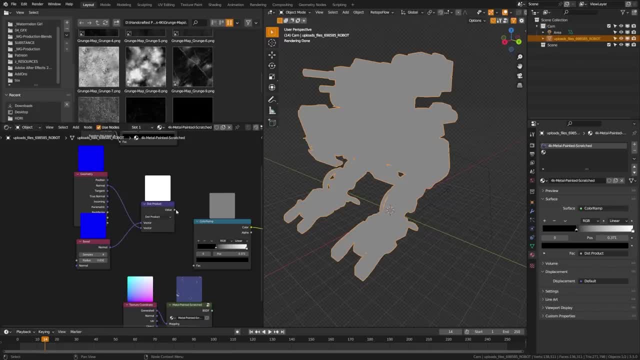 So we're going to go ahead and add another vector. So we're going to go ahead and add another vector. So we're going to go ahead and add another geometry node, And this time we're going to feed in the normals to the vectors and plug that into the factor. 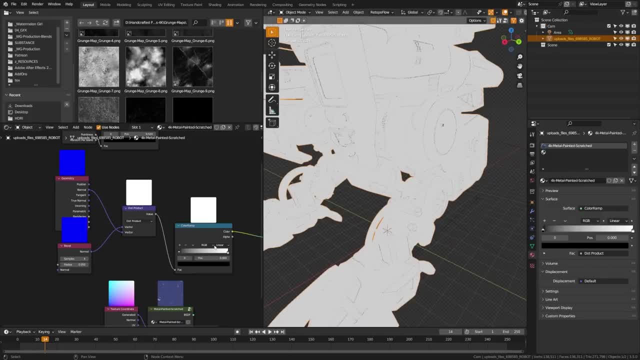 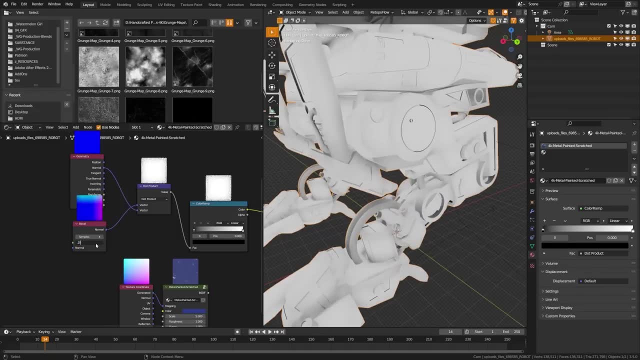 And now you can see that we get a much more refined option there, And this gets us kind of a much tighter node there, And then we can control the radius here, And I'm going to go ahead and set mine to something like 0.25. 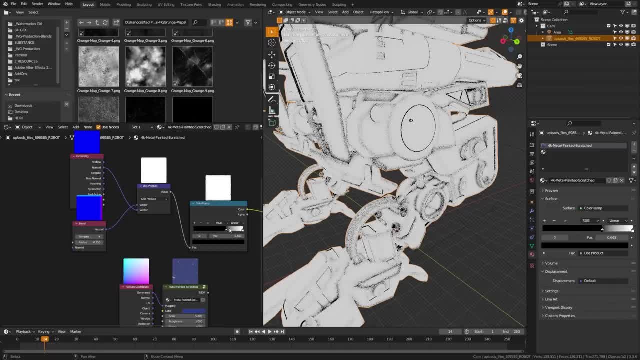 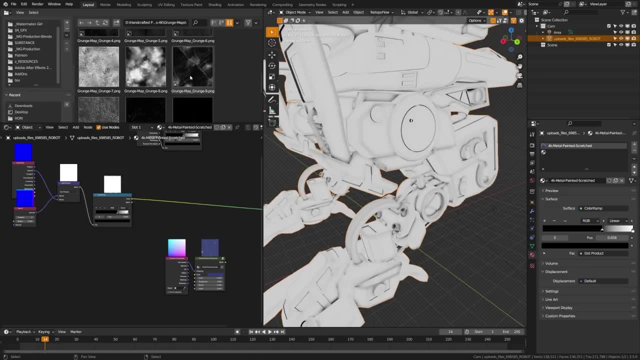 And you can see how that's starting to kind of get us some basic edge detection there. Perfect, Then what we can do is go ahead, And if we want to grunge that up, you can technically plug it into the radius. but you can also go ahead and plug it into the radius. 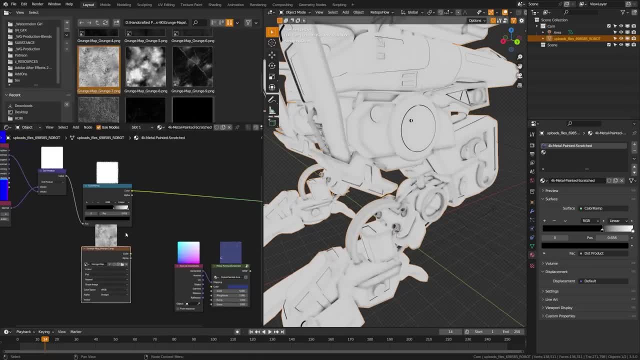 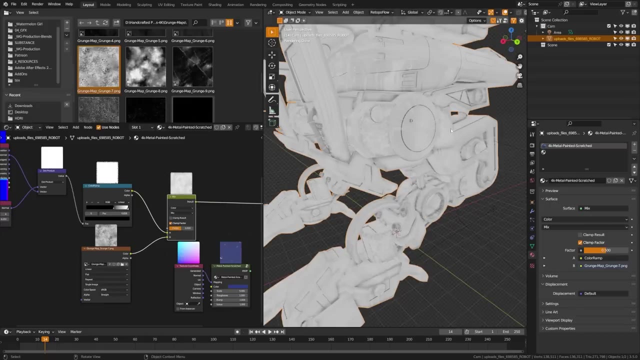 So let's go ahead and plug it in on a color mix node as well. So let's go ahead here, Add a color node, Plug this into the top here and plug this into the bottom and see what this looks like. You can see, now we're starting to get that color all over. 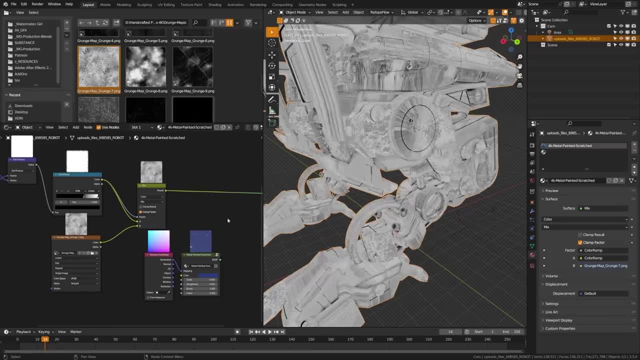 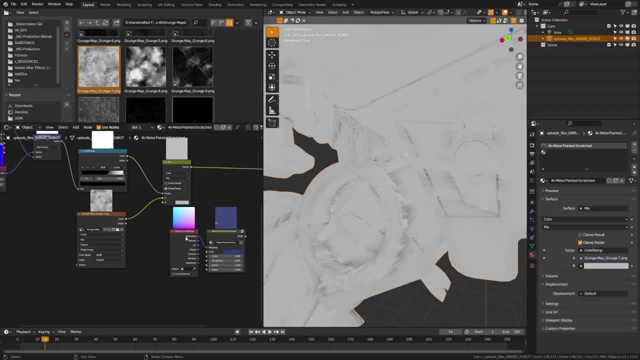 So we can go ahead here, Use this color as a factor And go ahead and switch these, And now you can see that we're only getting that data there, the bottom there, you can see that we're getting some stretch coordinates, so you can go ahead and. 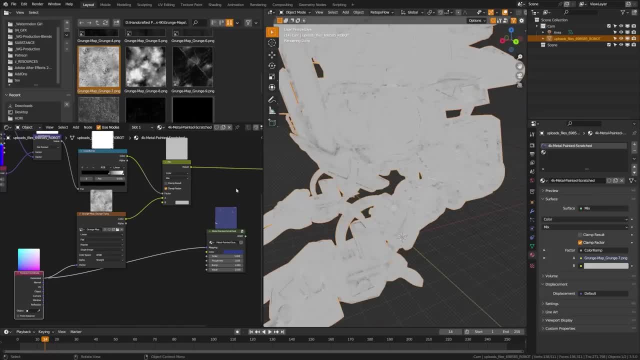 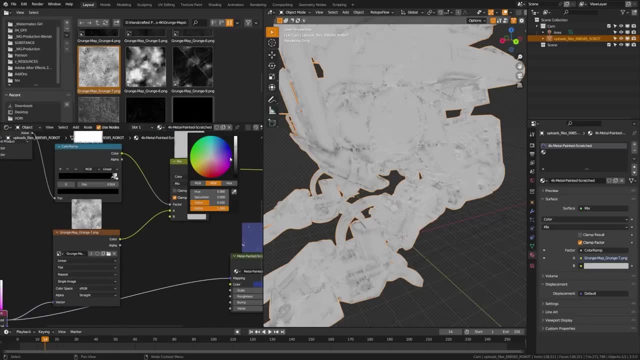 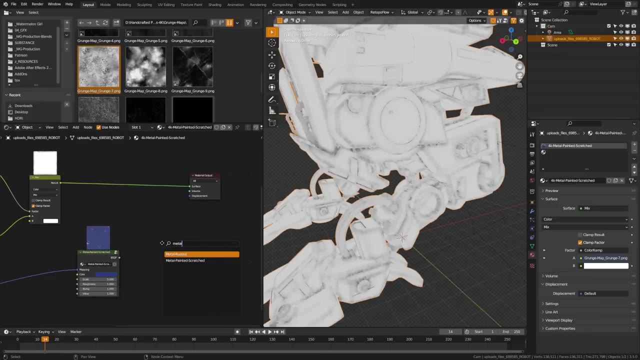 plug a generated coordinates in there and that'll help get you a bit better results. you can go ahead and crush that a bit more and get a few more of those edges perfect. then what we can do is we can go ahead and plug this into a mix shader. so if i go ahead and search here, i have a metal rusted. 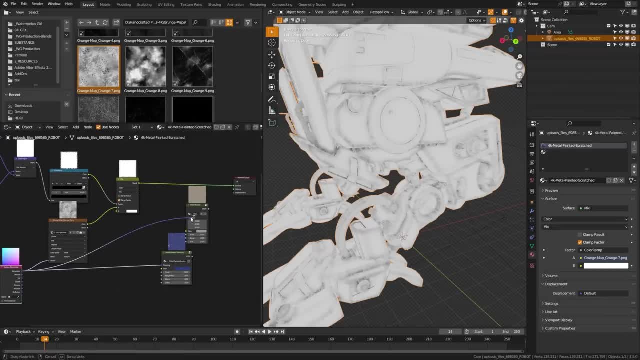 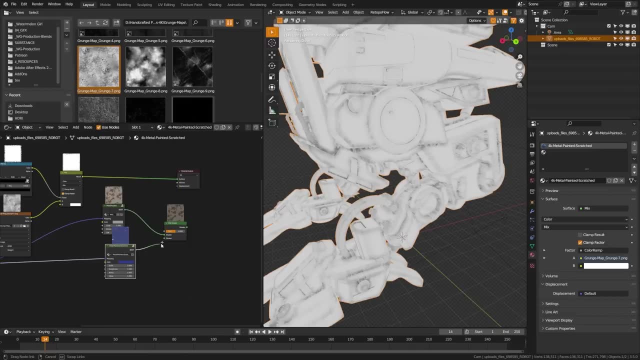 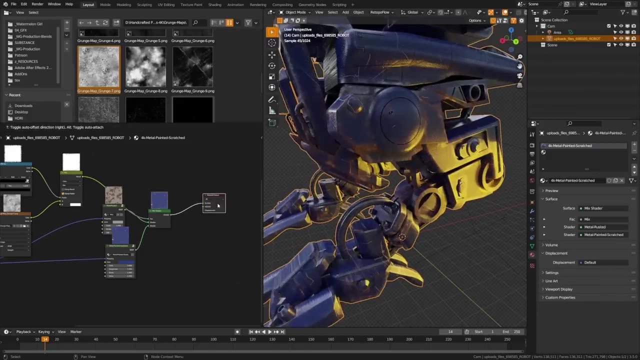 so i'll go ahead and use this as well. plug this into the mapping node there. we'll go ahead. plug this into a mix shader and then we can go ahead and plug our edge detect node in here and then plug this in for our final result. here you can see how we're starting to get a lot of wear and tear.